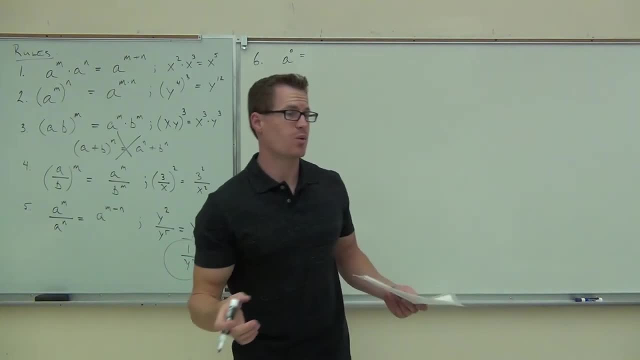 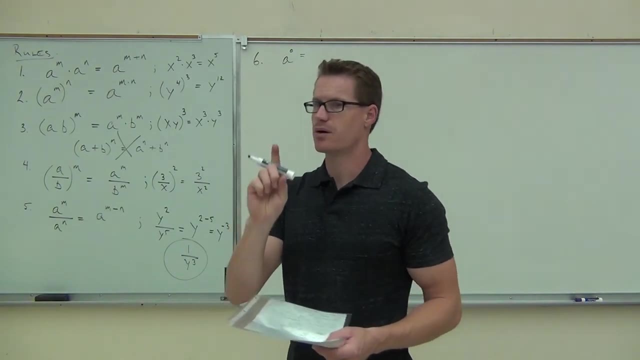 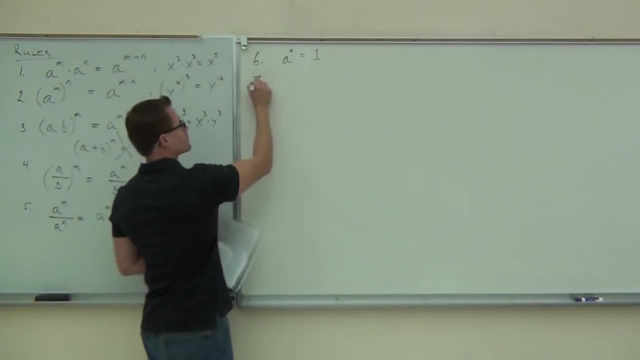 How much is that? Some people say zero, some people say one. What is it? It's not a cell, It's one. Yeah, it's one. Anything to the zero power is defined as one. And lastly, a refresher. 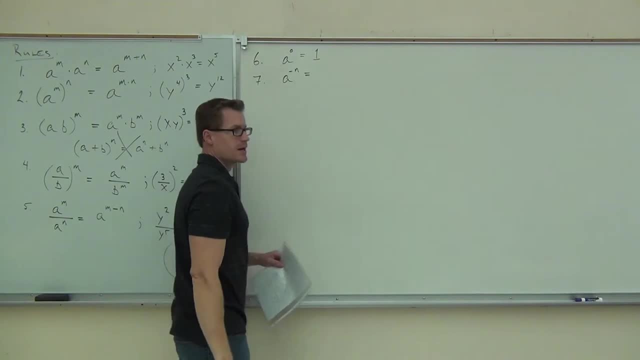 We did this last time. Just a good little note: to have Anything to the, The negative exponent, we can always change it to a positive exponent by doing what To the. So wherever it is, we change the part of the fraction that's on it. 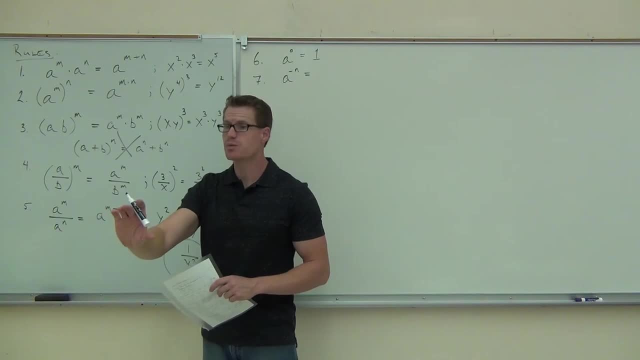 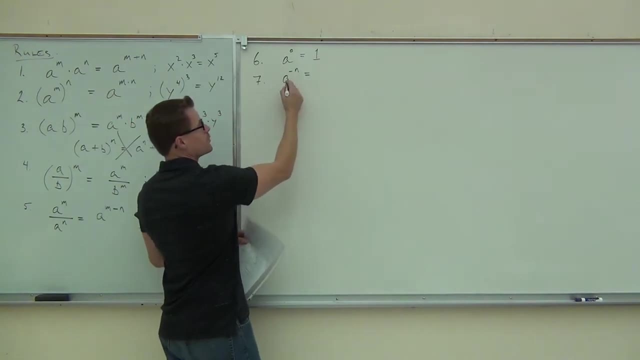 It's on the numerator and it's negative, we move it to the denominator, Because on the denominator we can make it positive by moving it to the numerator, We just change the spot of the fraction where it is. So, for instance, right here, we consider this to be. 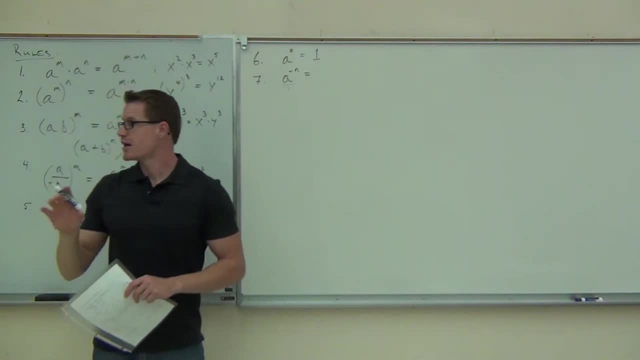 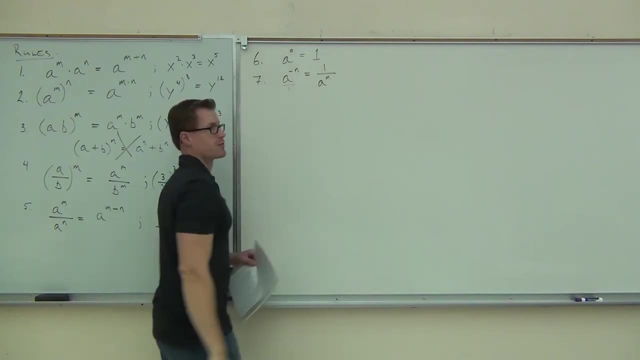 on a numerator, because you can write that over 1.. If we want to change the a to the negative n to an a to the positive n, what would we have to do Is we'd have to write this on the denominator of the fraction: 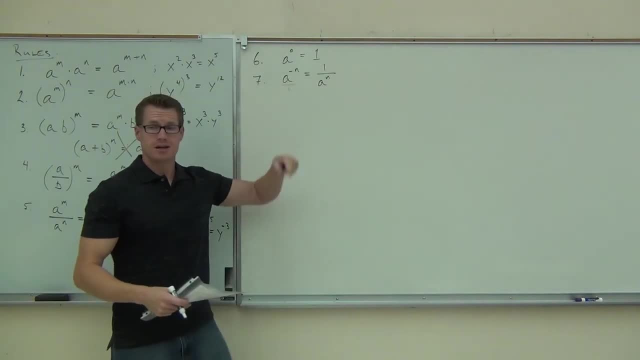 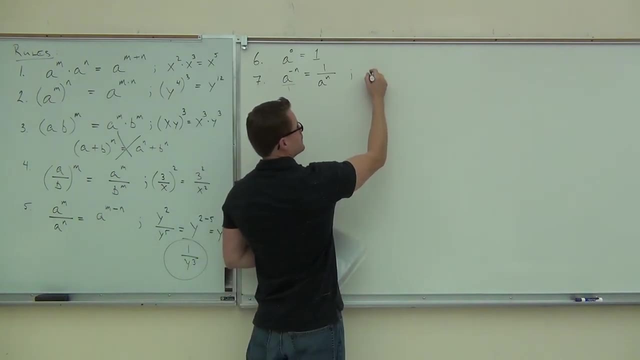 Remember, recall from last time, that it doesn't change the sign of the number, it just changes the sign of the exponent. And we did several examples, but I'll give you another one over here. Let's see X to the negative 4, we could write that as 1 over x to the 4.. 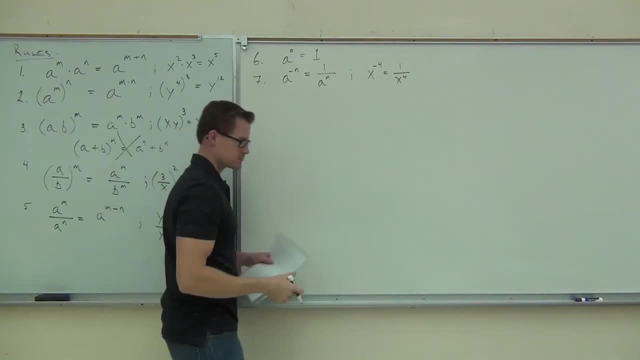 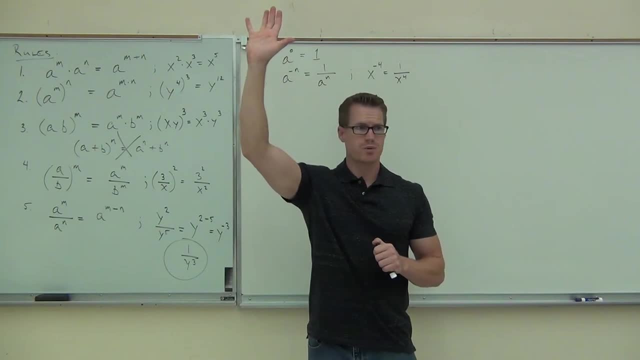 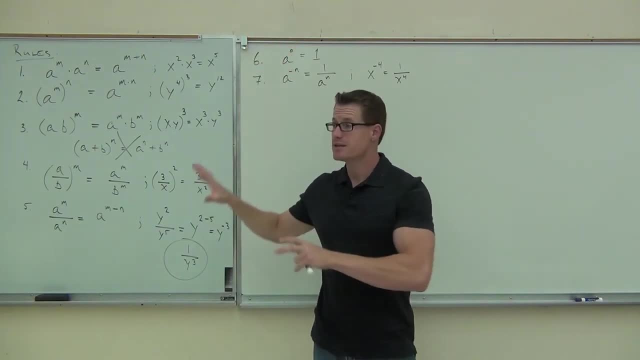 It should be a refresher for you. Now, what we're going to do is we're going to take these rules that we just kind of reviewed and we're going to apply them to our rational exponents. What you need to know is that every one- 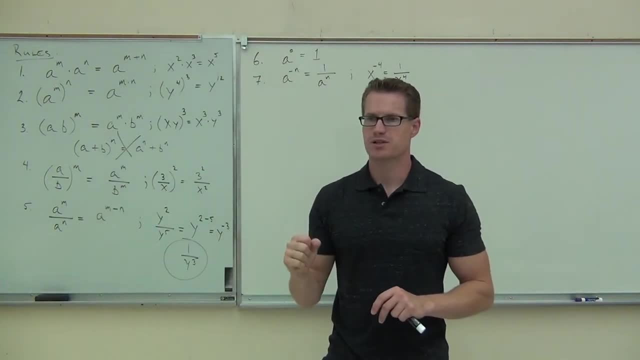 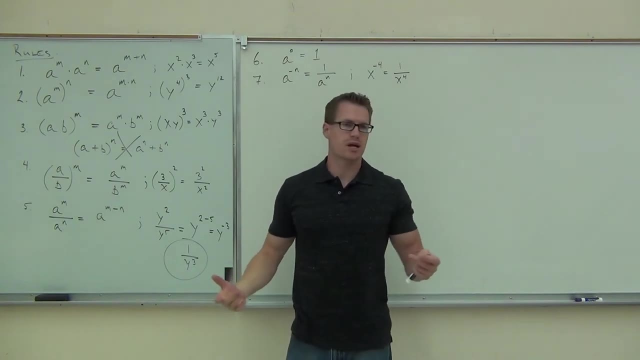 of these rules works exactly the same way for rational exponents as it does for whole numbers. Now I gave you some whole number or integer exponents, but right now I'm going to give you those fraction exponents. They work the same. 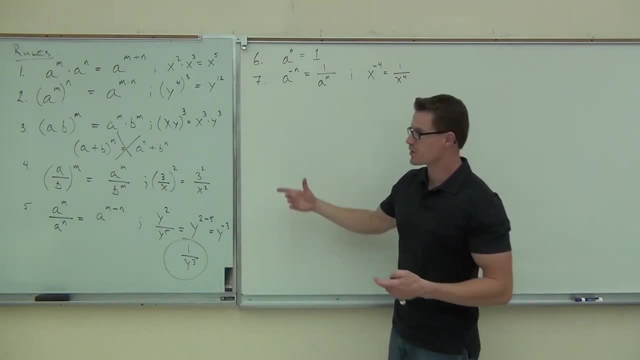 As long as you stick with these rules. there's only seven of them. Most of them are big, Very refresher. The only one that really might be a little new for is using this with those fractions, but it's the same ideas. 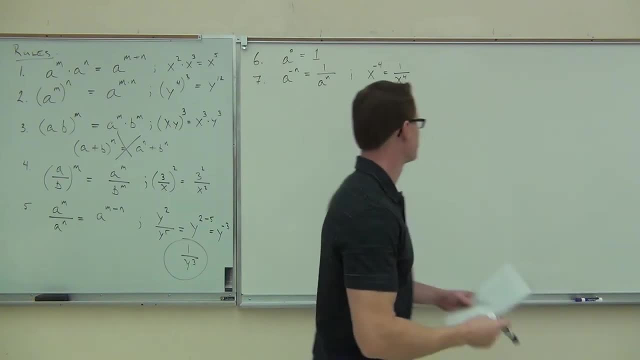 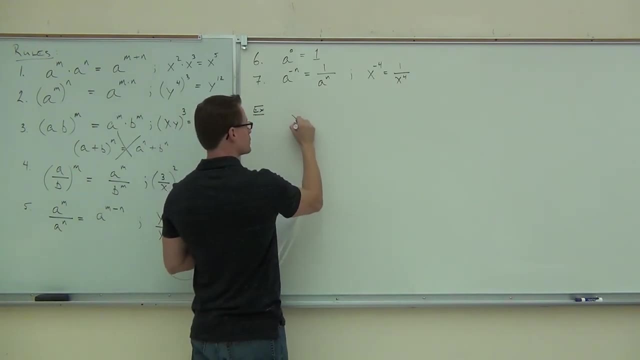 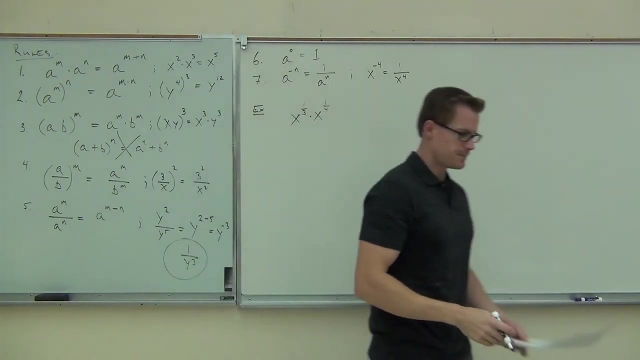 Are you guys ready to try some examples here? Okay, let's do that. Okay, we got x to the one third times x to the one fourth. That'sாwe're going to get, we're going to have, is a division. 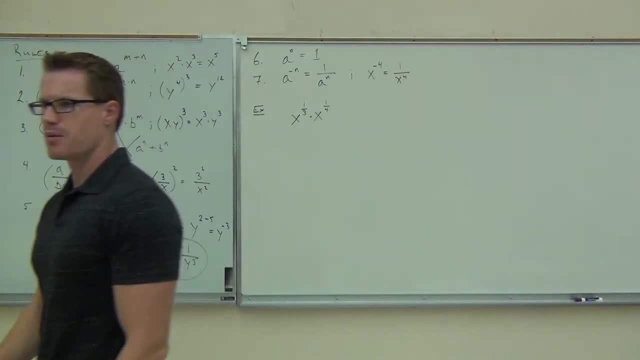 by operation of both fractions. that's a EXP. That's actually fine, Ladies and gentlemen. do we have a common base there? Do we have a common base? And they're being multiplied. So when we look at this, we're multiplying them. 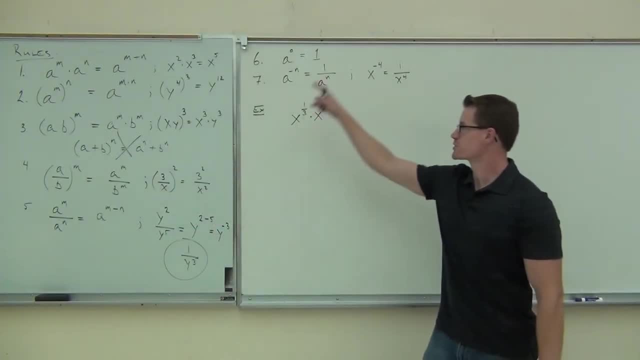 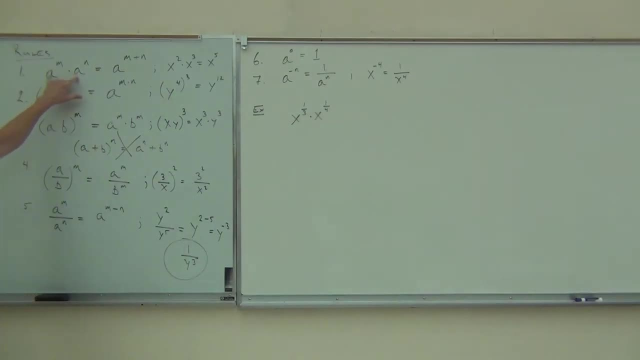 What situation are we most like? Rule one through seven. Which one are we most like, do you think? Rule number one. I've got two things with a common base that are multiplied together and I have some exponents up there. So what am I going to do to those exponents? 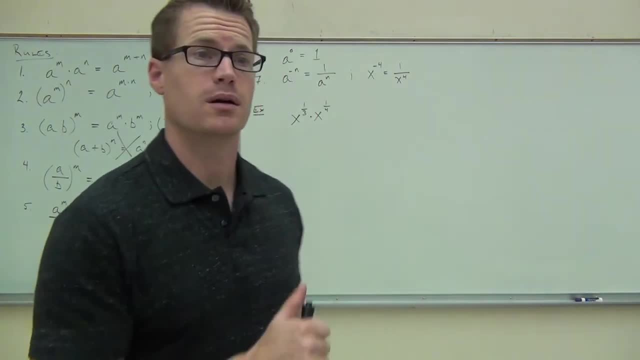 Am I going to add them, subtract them, multiply them or divide them? What do you think? For sure, I'm going to add them. That's what that says, right? You know what a lot of people do? A lot of people do this. 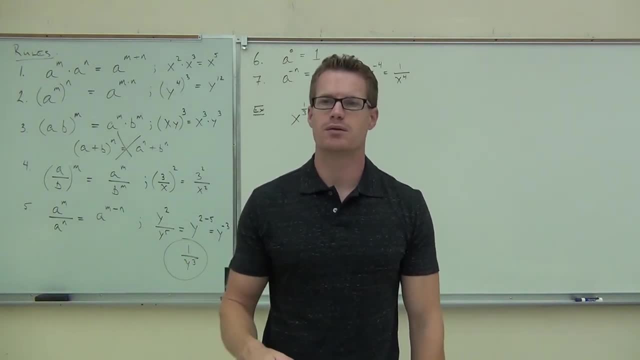 They make the mistake- and they're doing this really quickly because they get the handle on it right, but then they're really not reviewing it enough and they get to the test and they go- oh, that's x to the 112th. 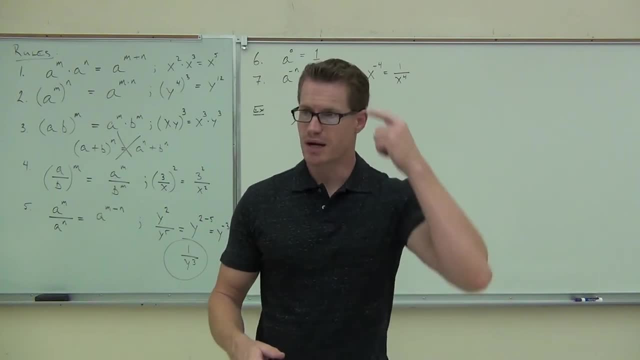 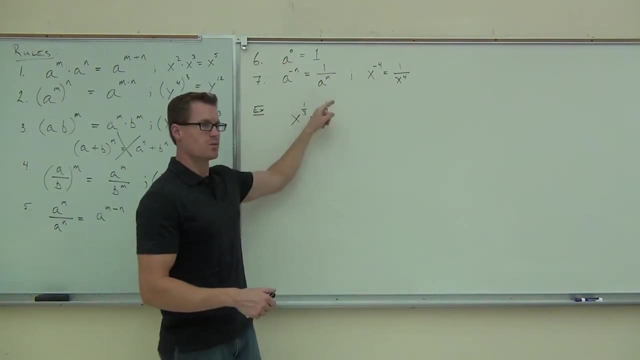 Do you see how easy that is to do. If you're just thinking multiplication, your head's thinking multiplication, right, You're not thinking really the exponent rules. if you're just seeing this, If you just see this, you go: oh, 112th, yay, I'm done. 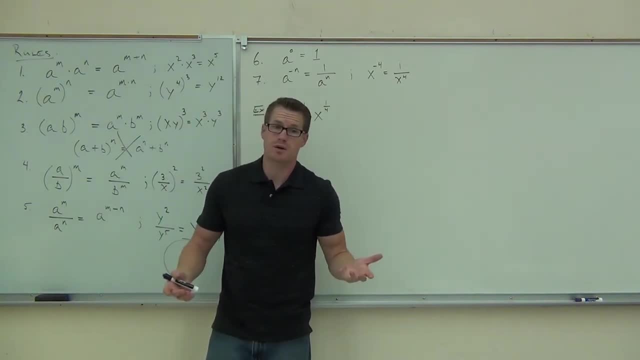 Well, if we do that, we're kind of missing the big picture here. right, These are exponents And exponent rules. say, if I multiply on a common basis, what I'm really doing is I'm adding those exponents together. That's what I'm really doing. 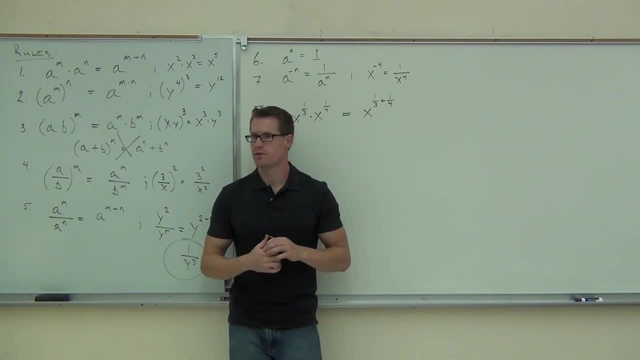 Now can you add one-third plus one-fourth? You do. We don't have to add fractions, right? This is a fraction class. We're past fraction class, It's great. So if you use your calculator, I don't care if you use your calculator or do it off to the side- 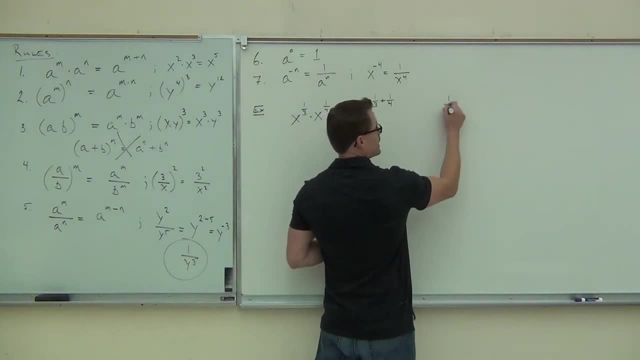 I would personally do this off to the side. I'd just say, okay, I know I need it. Add one-third plus one-fourth. That means a common denominator. A common denominator is going to be what? So we're going to multiply this by 4 over 4.. 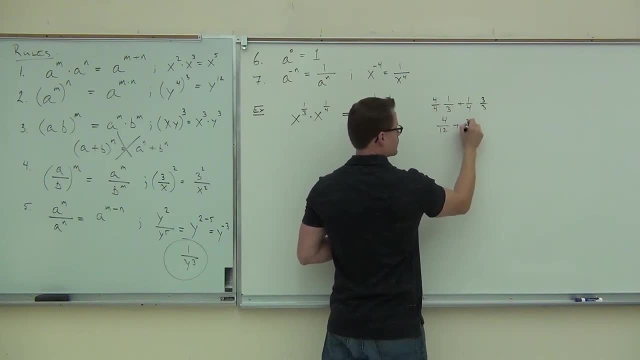 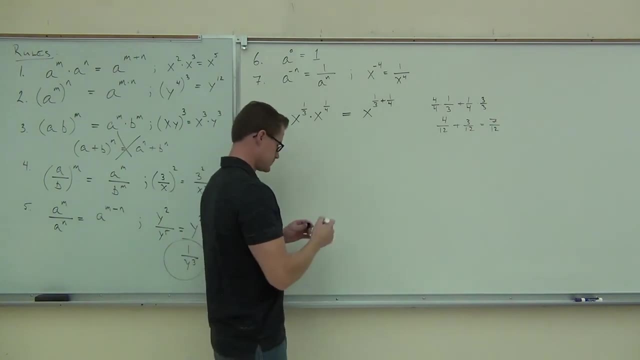 This by 3 over 3, we'll get 4 twelfths. We'll get 3 twelfths. That's going to give us 7 twelfths. So instead of x to the one-third times x to the one-fourth. 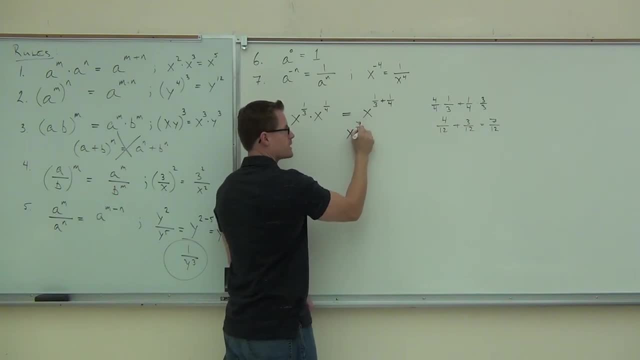 or x to the one-third plus one-fourth. we actually added those and we got x to the 7 twelfths. Are you okay with that one? Yeah, Hey, by the way, could you write this as a root? 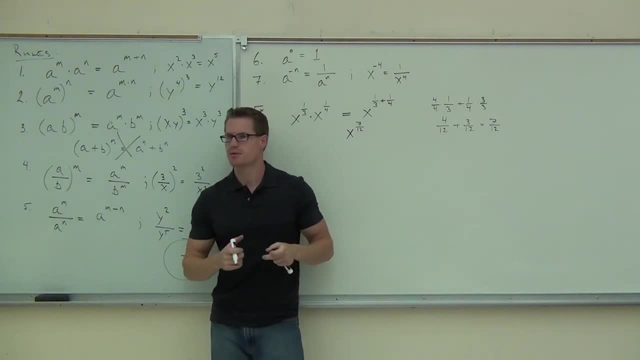 No, Could you write that as a root? What type of root do we have? Twelfth root. Twelfth root of what? x to the 7 twelfths. So, if you wanted to, if the problem asks for a root, 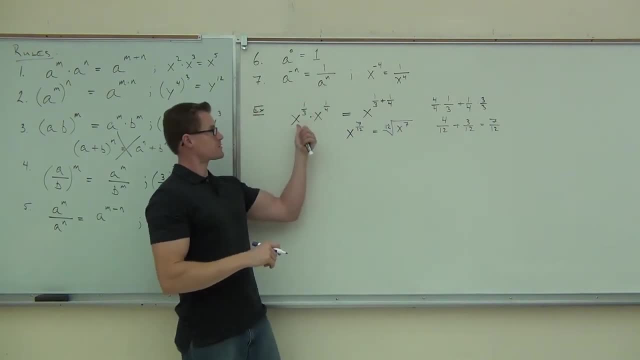 that's that root. These things are the same thing, So this actually makes that. I want you to see how this works. This stuff actually works here. Notice that the common denominator- the common denominator- is the root, isn't it? It is the root because we know that the denominator makes the root up. 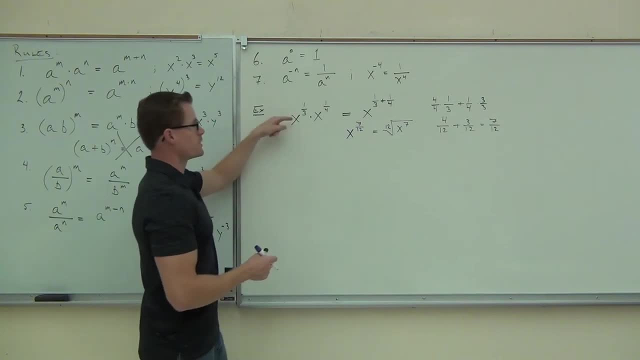 so when you find the common denominator, that's making a common root. This you could have written as a q root of x, right. This you could have written as a fourth root of x. Multiply those two things together, you have to find a common root. 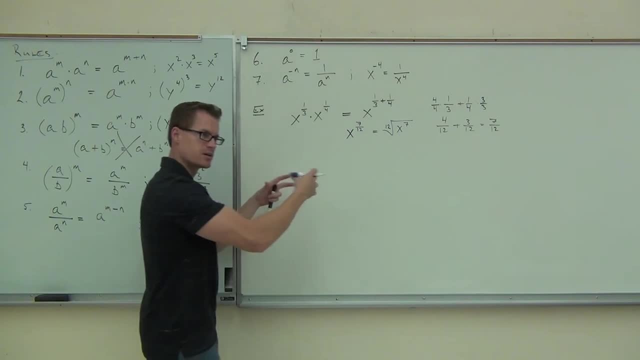 In that case it means a common denominator. That's why all this stuff is intertwined. It works like that. All right, let's move on here Before I do. are there any questions on that example? Because this is just our start-off point. 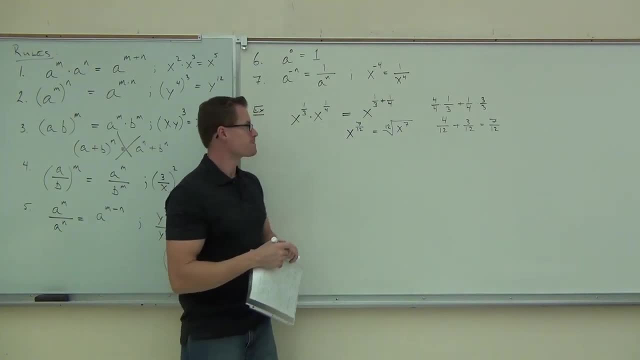 Are you guys all right with that one? So the final answer is the square root. If it asks for the root, then yeah, that's the final answer. If it doesn't, you can definitely leave it. X to the 712th. 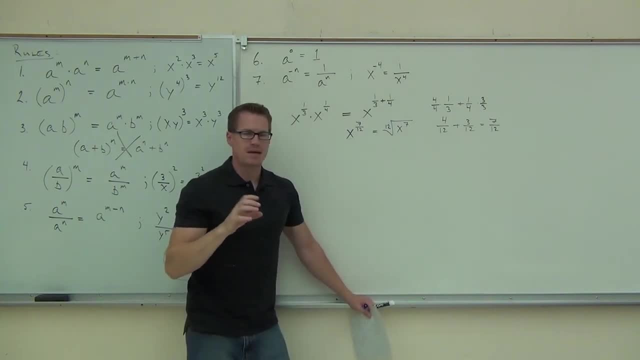 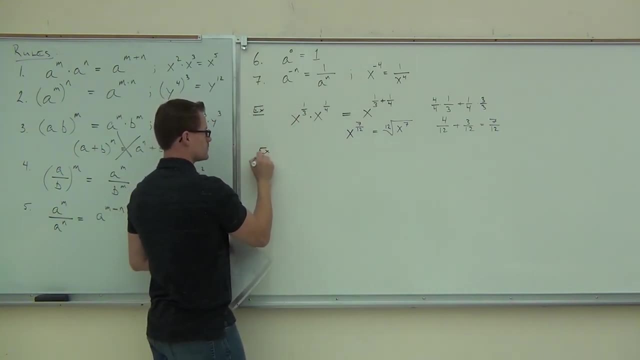 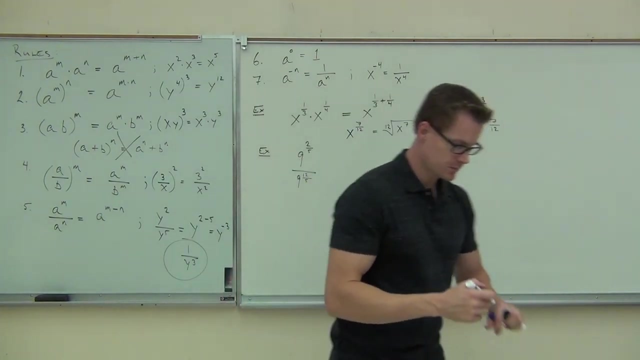 You don't have to do this. What I'm trying to do is make you remember that this is possible. I don't want you to forget this. 9 to the 2 5ths over. 9 to the 12 5ths. 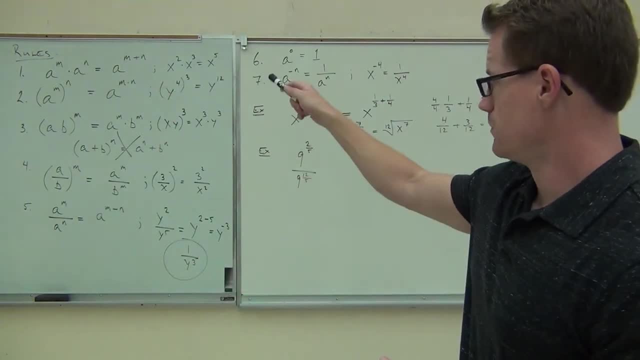 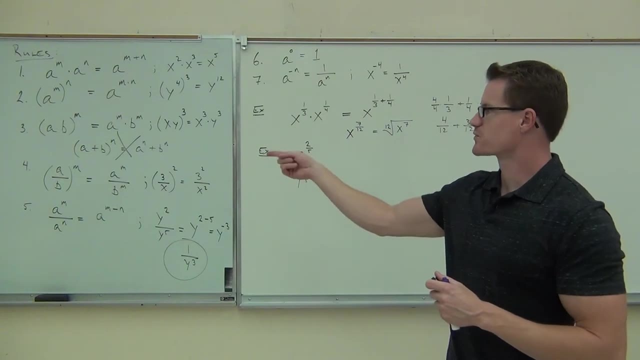 Hey, let's look back at our rules. Can you tell me what rule we most like, 1 through 7.. There's only two that have fractions right. There's 4 and there's 5.. The 4 would be everything raised to a power. 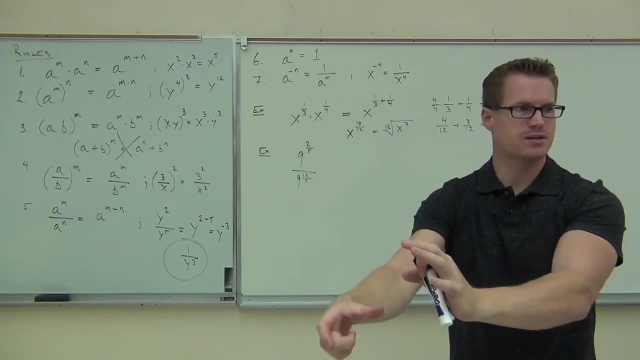 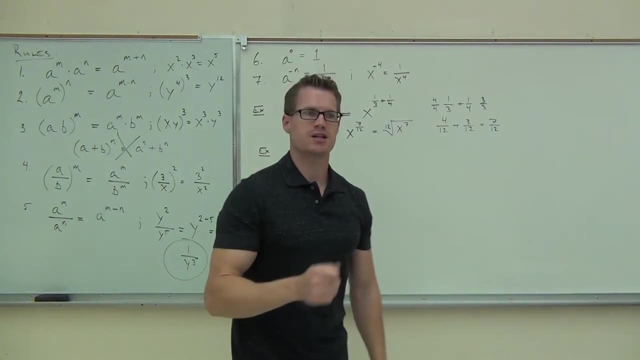 We're not there. We're actually at number 5, where we have something raised to a power And something raised to a power. we have the common base there. You with me on that? that's 5? Okay, so what are we going to do with those exponents? 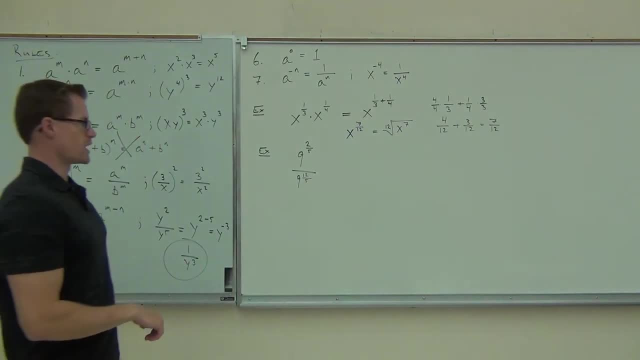 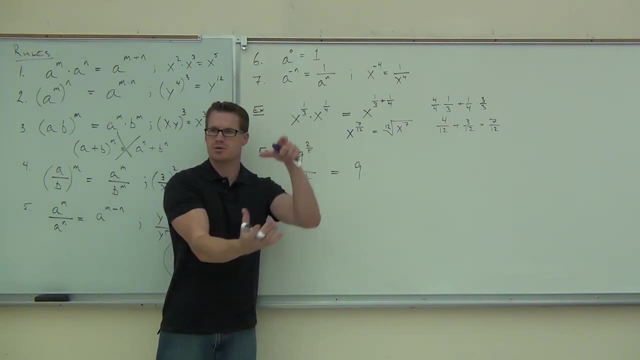 Add, subtract, multiply, divide. What do you think Definitely subtract. What we do in this case is we take our 9.. We write only one, 9, because we're combining the exponents. We're combining these two things by subtracting exponents. 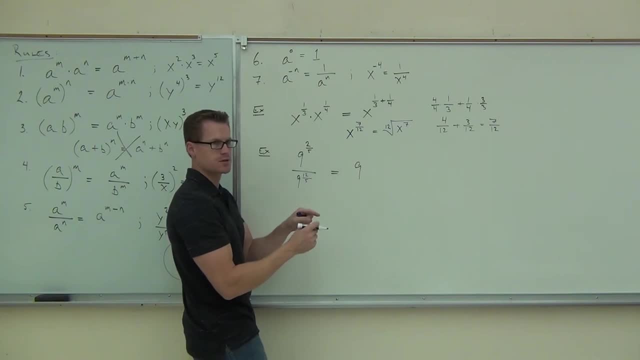 Are we going to have 12 5ths minus 2 5ths or 2 5ths minus 12 5ths? Can you do 2 5ths minus 12 5ths? That's kind of better than that problem, right. 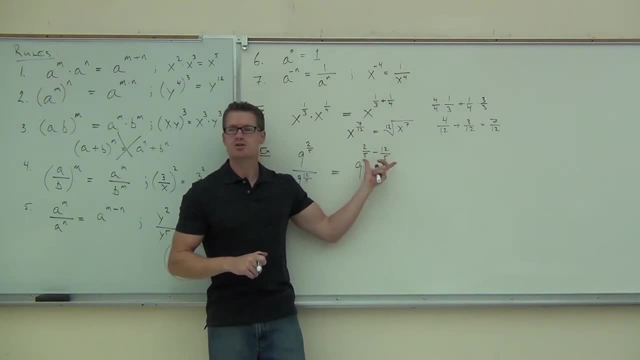 You don't even need a common denominator, It's already there for you. That's great. How much are you going to get? 2 5ths minus 12 5ths Negative 10 5ths- It's negative. 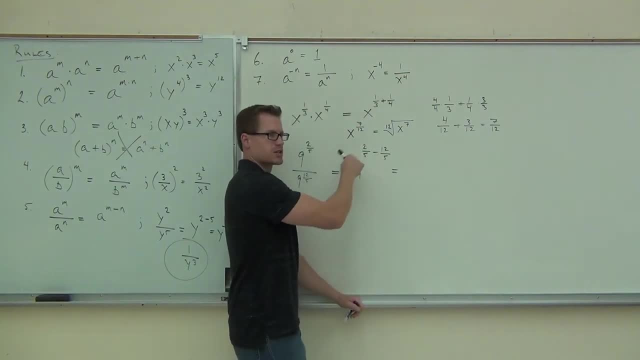 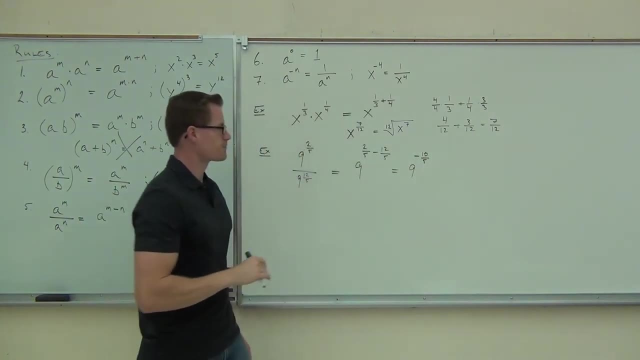 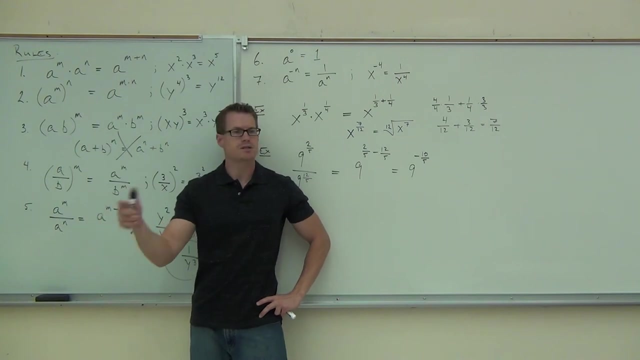 Okay. Is the number negative or just an exponent? It's an exponent. Negative 10: 5ths. Are we done? What do we need to do? Negative 10, negative 2. This is a fraction. Even though it's an exponent, it's still a fraction. 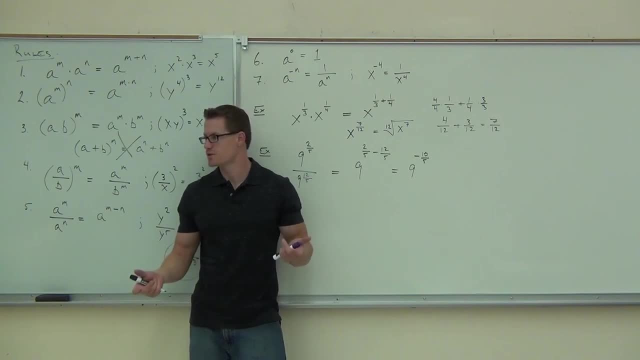 which means that you can simplify it just like you would any other fraction. So negative 10 over 5, we need to know that's negative 2.. I'm not going to give you negative 10 5ths. I don't want that. 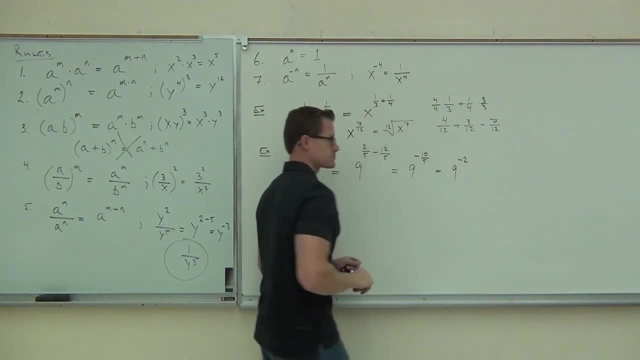 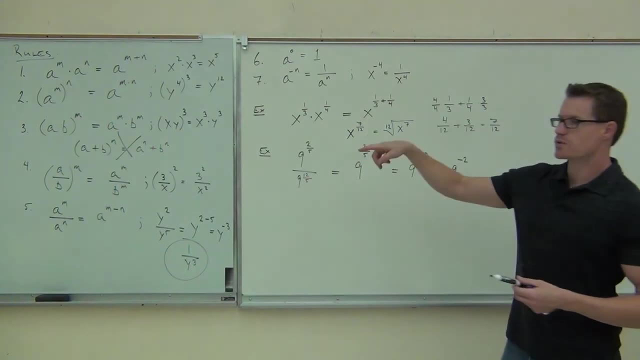 We say, oh okay, that's 9 to the negative. 2. Tell me another thing we can do with that. How do I write 9? You're positive? This is another rule. What rule is this? 7. 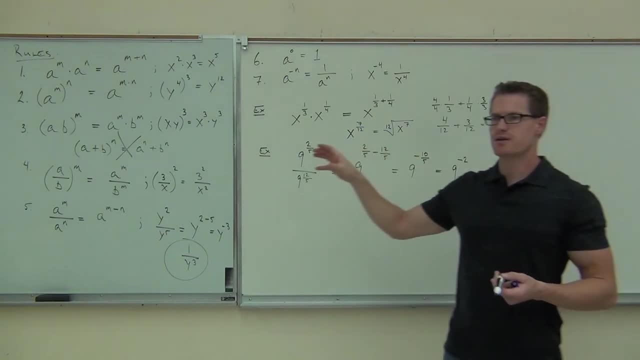 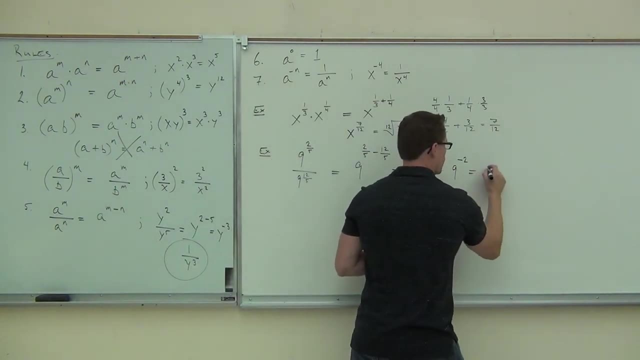 That's number 7. It says: okay, anything that's raised to a negative exponent, we can make that a positive exponent by putting that on the denominator of a fraction. So right, here we're going to go. all right, I want 1 over 9 squared. 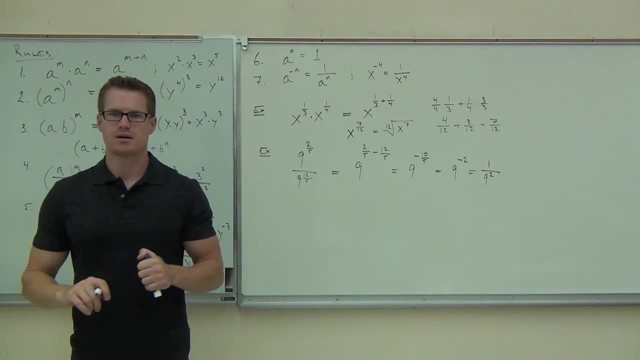 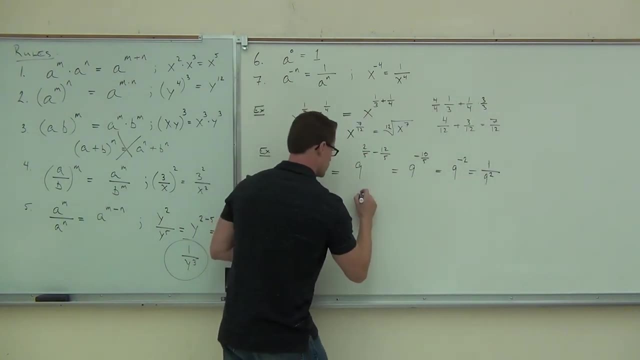 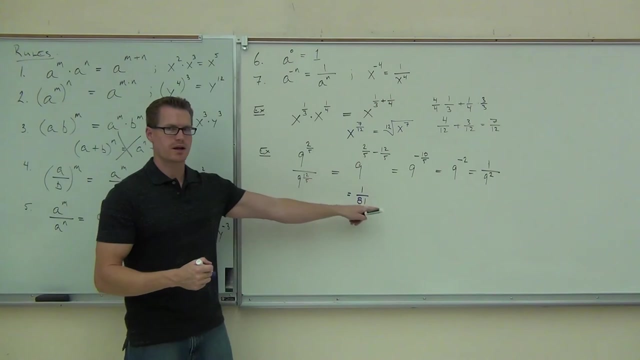 1 over 9 squared. Ladies and gentlemen, how much is 9 squared? So this is 1 over 81.. 81. Gee, so we worked this all the way down. We only got 1 out of 81.. 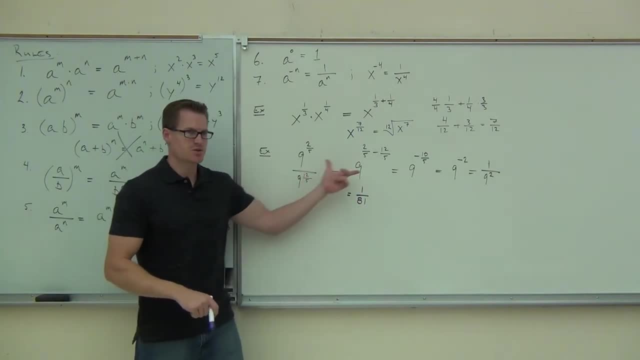 Isn't that kind of interesting that this means the same thing as that Just by using our rules and manipulating that, we get that down to 1 over 81. It's kind of cool, right? That's a whole lot easier to think about than that. 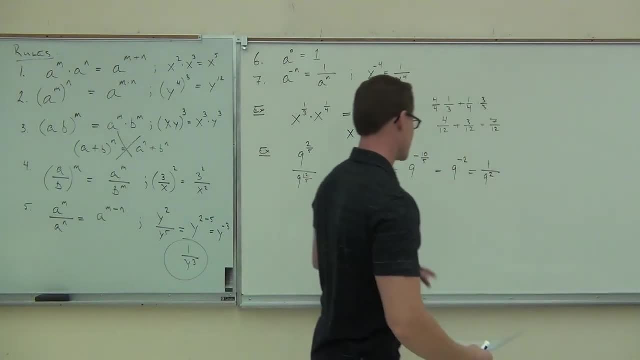 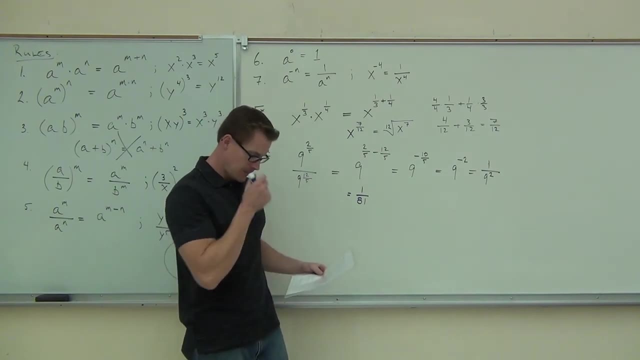 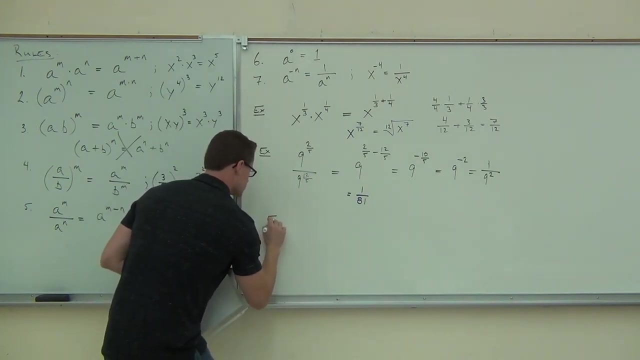 Can you go back to the original problem? You can, but I mean, it's after you do all this. if you just looked at this, there's no way to tell that that's what you started with. Yeah, Let's look at it again. 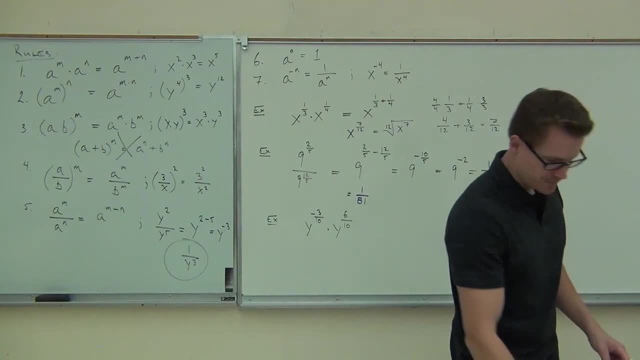 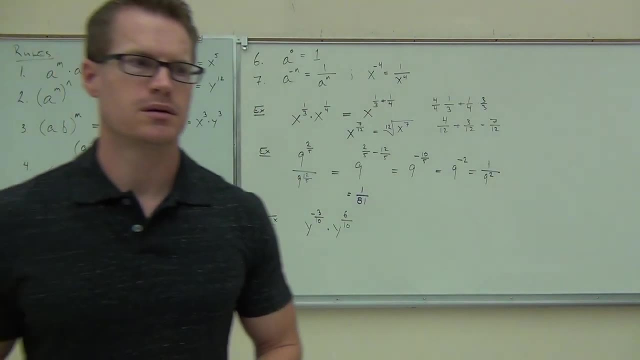 y to the negative. three-tenths times y to the six-tenths. Hey again, what situation are we? Let's look closer at the board. What one are we? What do we look like here? Well, we're still at number 1.. 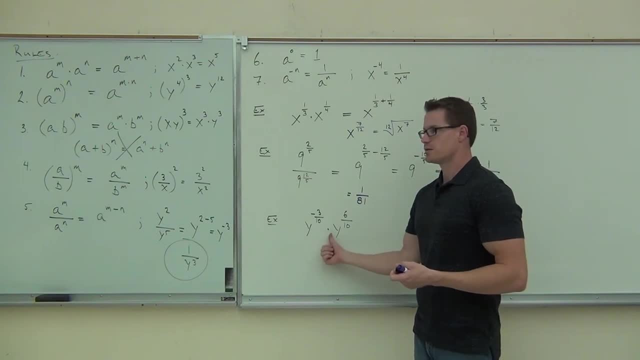 We've got common bases. We're multiplying. That's definitely number 1.. What are you going to do with these exponents? folks Add them. You can add them. Even though one's negative, that's okay, You can still add them together. 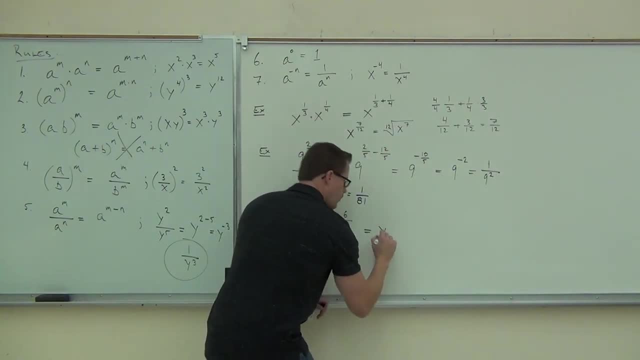 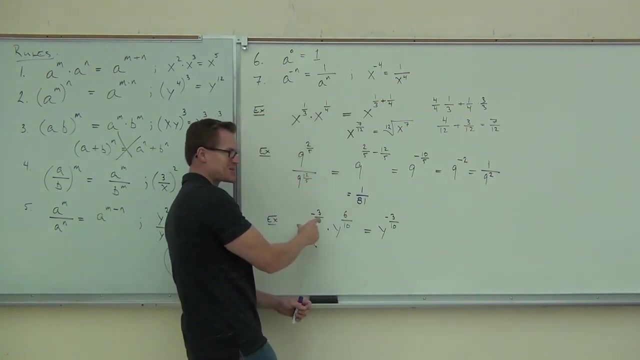 That's fine. So we know we're going to have y to the negative 3 tenths times y to the 6 tenths. I just wrote the same thing twice. Since we have those common bases, we're multiplying. We know we're going to add the negative 3 tenths and the 6 tenths. 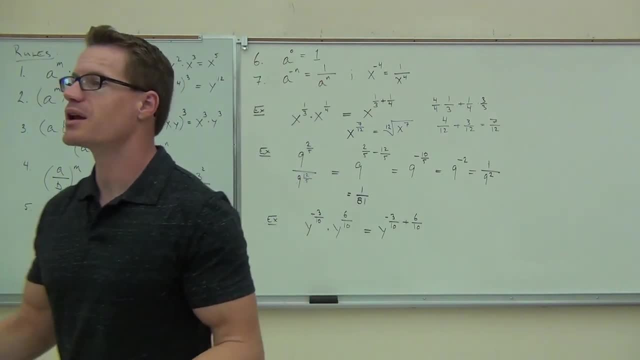 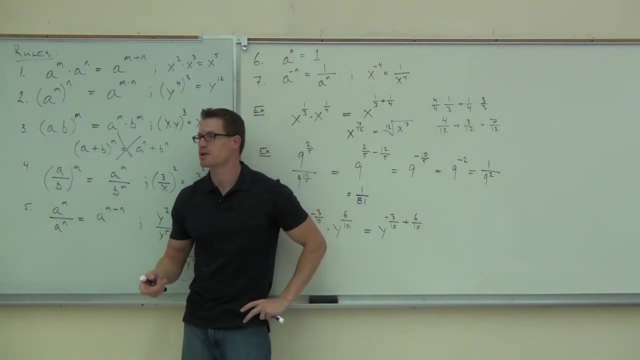 What's great is we already have a common denominator. If you don't have a common denominator, you've got to find one. if you're adding fractions, That's what we did in this first example. But now that we have negative 3 tenths plus 6 tenths, how much are we going to have? 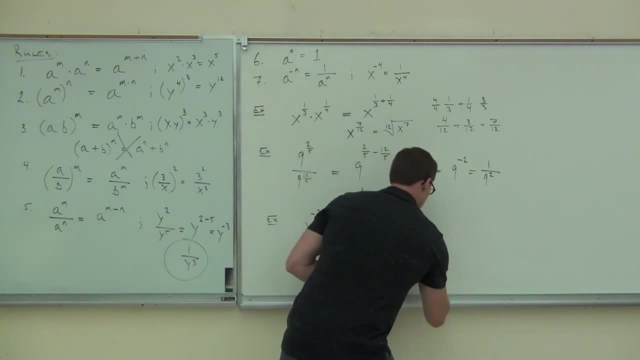 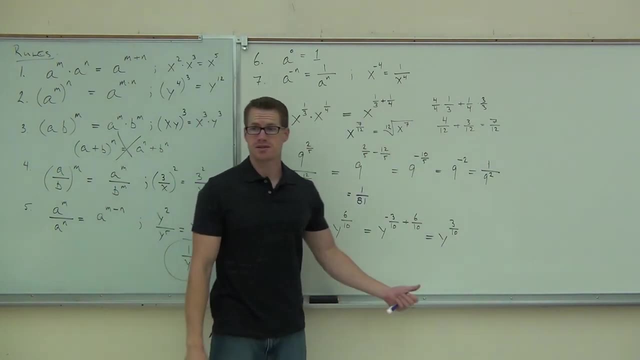 3 tenths: Positive 3 tenths. Okay, very good, Add those together, You get 3 tenths. Could you write this as a root? Yes, 10th root. Good, yeah, 10th root, because that's our denominator. 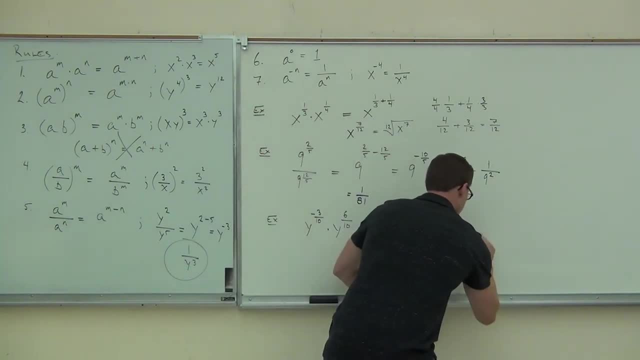 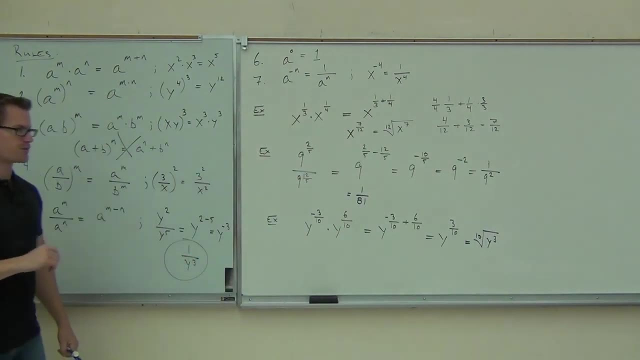 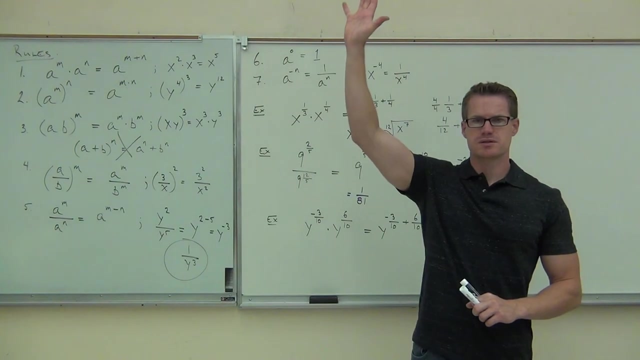 And the power is the numerator. so we would have that exactly. That's as far as we could go. Would you raise your hand if you feel okay with these ones? so far, All right. We're going to try a couple more together. 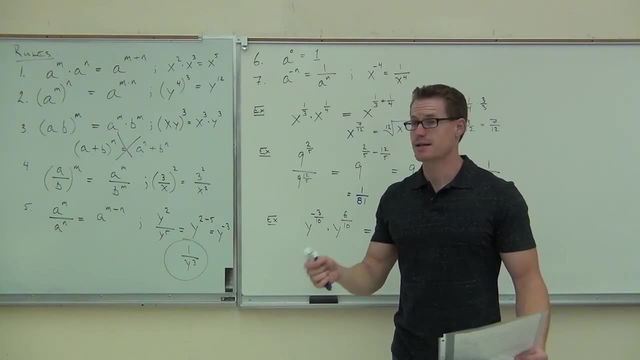 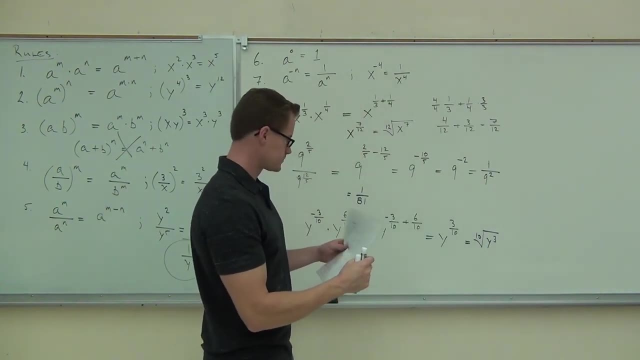 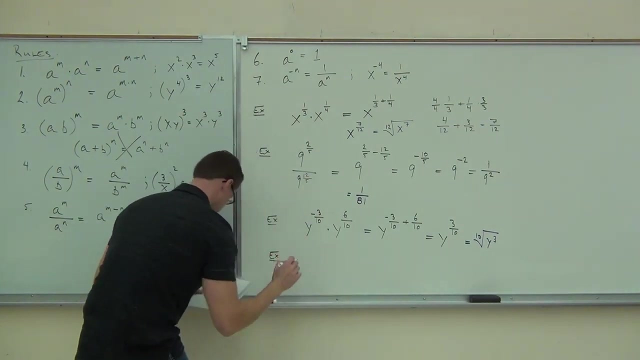 I'll give you several to do on your own. I want to make sure that you guys can do this. Then I'll move on and I'll show you how we can really apply this to some unique ideas. 11 to the 2 ninths. 2 to the 3 tenths. 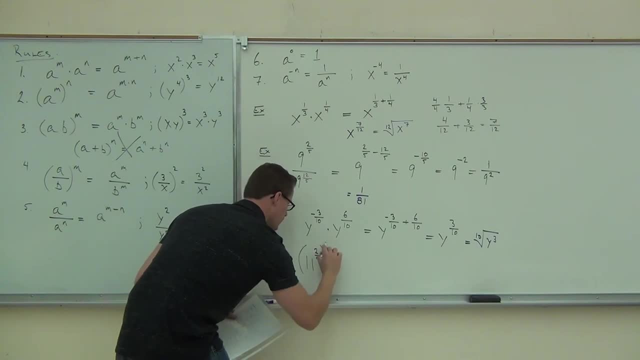 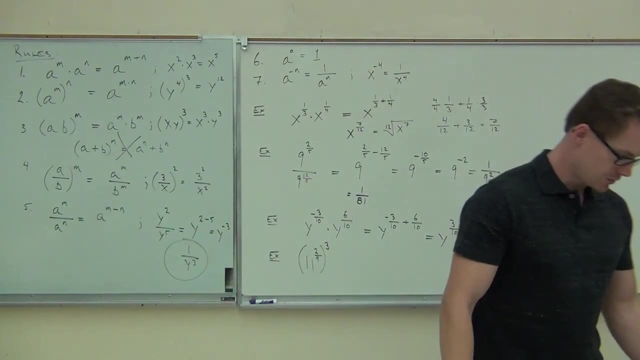 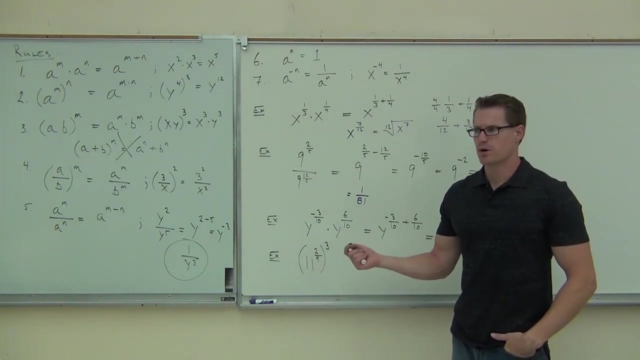 11 to the 2 ninths, 2 to the 3 tenths- the third power, Eleven to the two ninths, all raised to the third power. What do you think about this one? What rule are we for that Number four? Number four would be a. 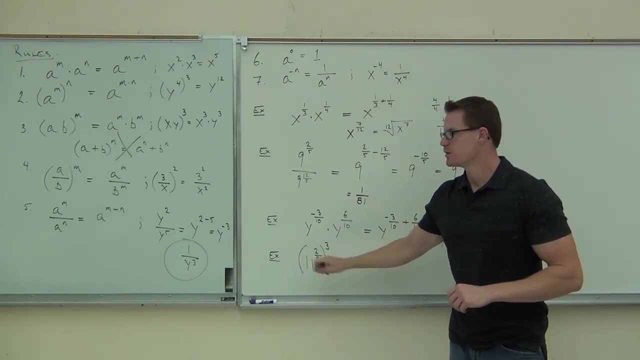 fraction raised to an exponent. We don't really have a fraction. We have. that's an exponent, right, And that's an exponent Which one is that? That's number two. That's right. This says an exponent raised to an exponent with some number or some value. We have some value. 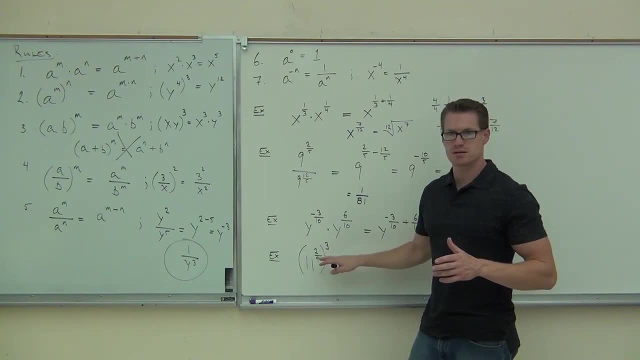 We have an exponent raised to an exponent. Do you guys see it? Yeah, How come you don't have a third power to the base? This one to this one? Yeah, You are. You are, because what you're doing here is this means eleven to the two ninths. This would be eleven to the. 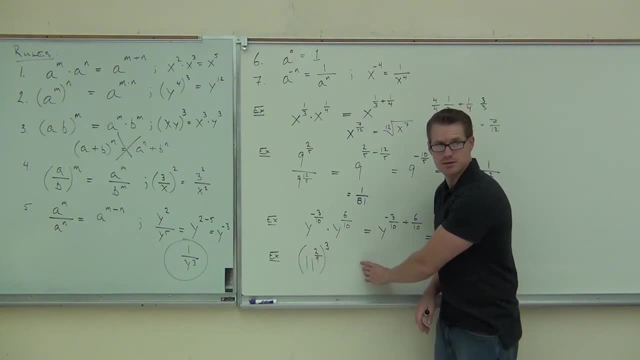 two ninths times eleven to the two ninths times eleven to the two ninths. Does that make sense? Yeah, And when you do that, you're going to have a third power to the third power. Yeah, And when you do that, you don't multiply the elevenths. They're already being multiplied. 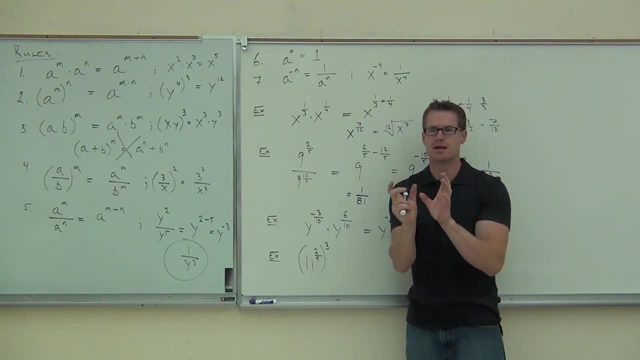 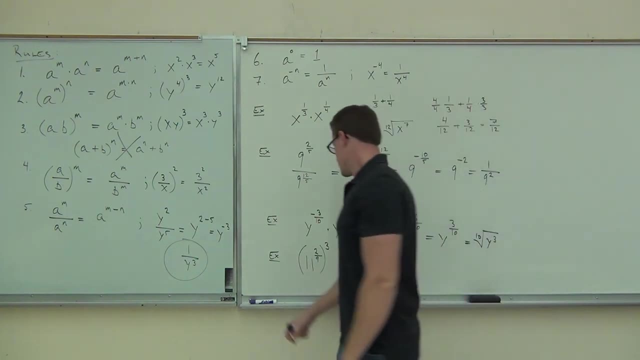 You're taking those exponents and you're making it so that you don't really have to deal with the elevenths. You're dealing only with the exponents. Indirectly, you are dealing with the elevenths. Does that make sense? You are doing that. Okay, eleven to the two ninths. 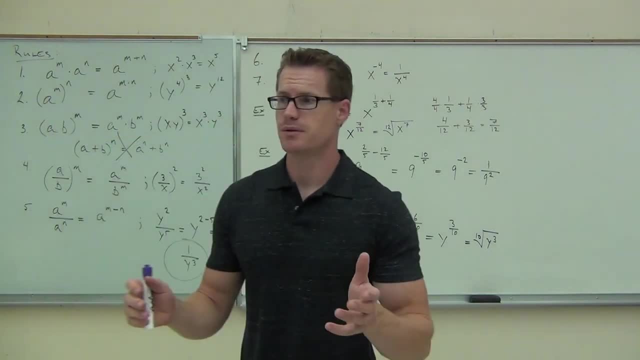 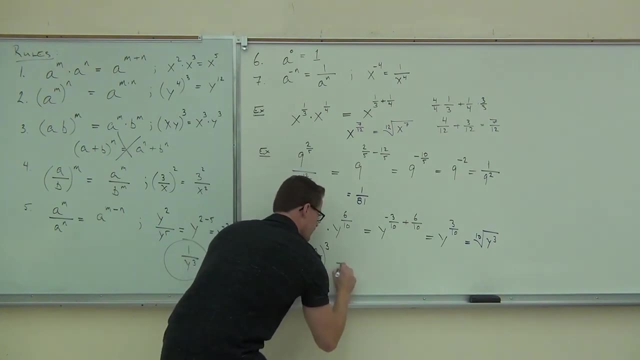 to the third power. What are we going to do with those exponents? folks, Definitely multiply them. Yeah, we have an exponent raised to an exponent there, So we're going to have sure, eleven is still our base. The base is still our base, So we're going to have eleven. 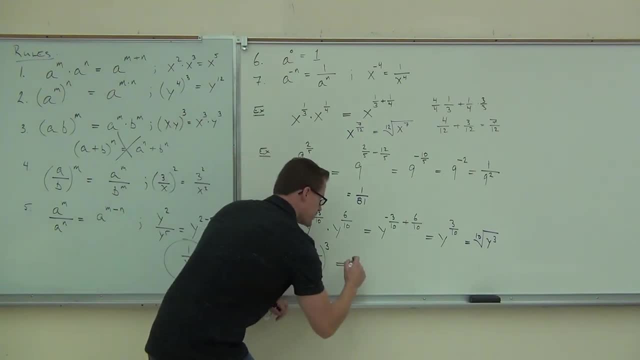 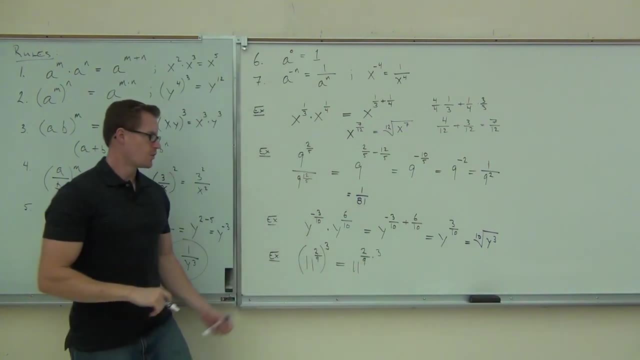 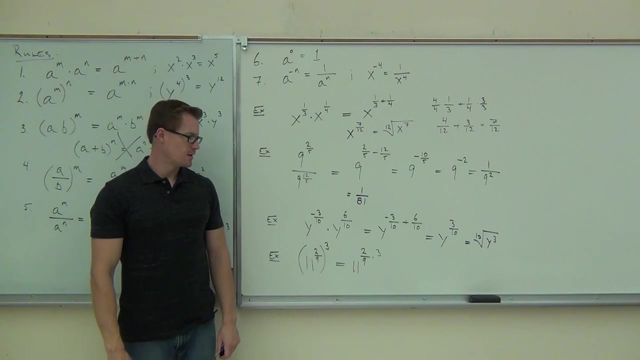 to the fourth power. The base doesn't really change when you're dealing with exponents, But up here for our new exponent, we'll have two ninths times three. We're multiplying those exponents. Yes, no, No, Okay, How, What are we going to get?